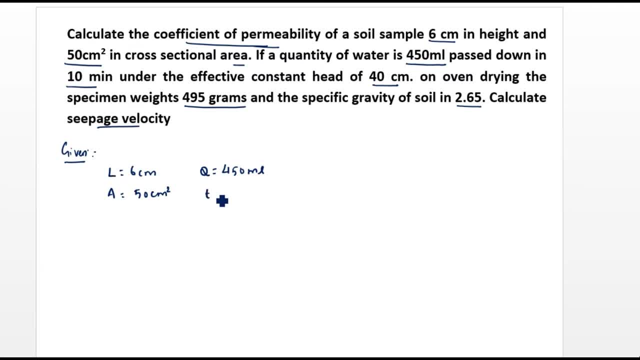 So then time T equal to 10 minutes. So 10 minutes that's given, So that is 600 seconds. Next H, small h equal to 40 cm. So that is constant height method. So constant height is 40 cm. So then mass equal to 495 g. 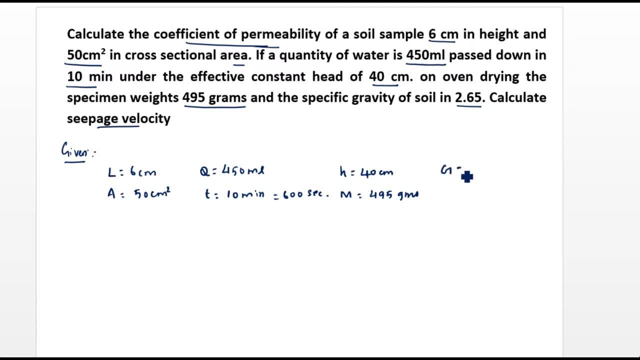 So then, specific gravity is given 2.65.. Okay, so now we have to find out the coefficient of permeability. So the formula for the in the constant height method, the formula for coefficient of permeability. So K is equal to Q into L divided by ATH. 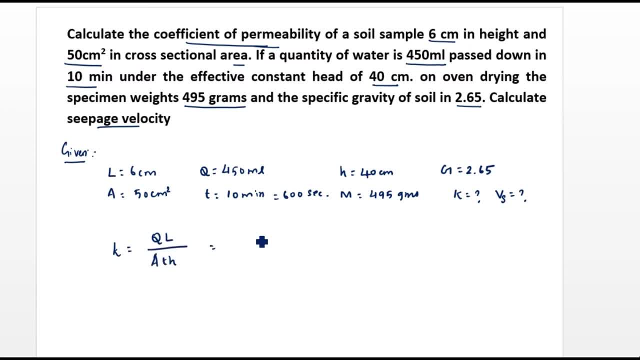 Okay, so we can directly substitute all the values over here. So the Q is 450 ml into. so then the length is 6 cm divided by so the area is given, That is 50 ml. one that is 50 centimeter square into time is 600 seconds into H with the. 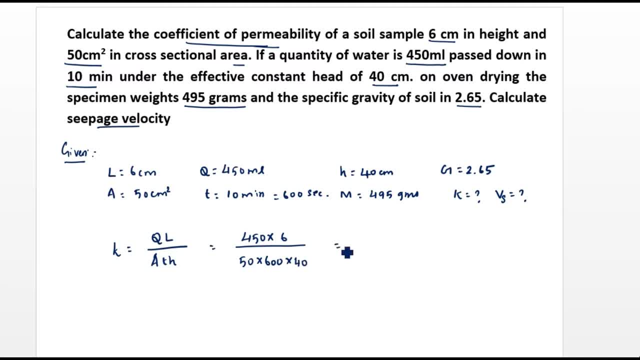 value is 40 centimeter. okay, so we can substitute all the values. we got the value answer 2.25 into 10 power minus 3 centimeter per second. okay, so we find out the first question answer. so, second thing, we have to find out the seepage. 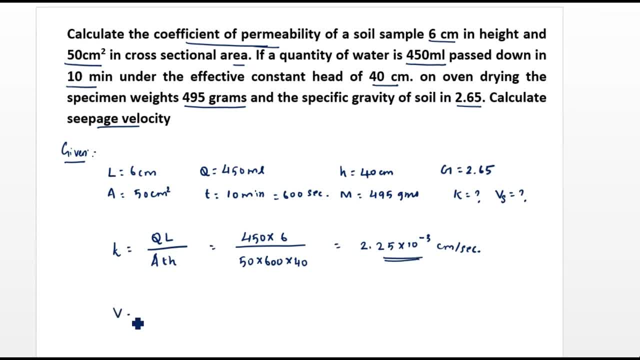 velocity. so now this V equal to capital Q, divided by A into T, so Q is 450, that's a given. divided by area, also given 50 into time, is 600 seconds. okay, so now we got the value 0.015 centimeter per second. 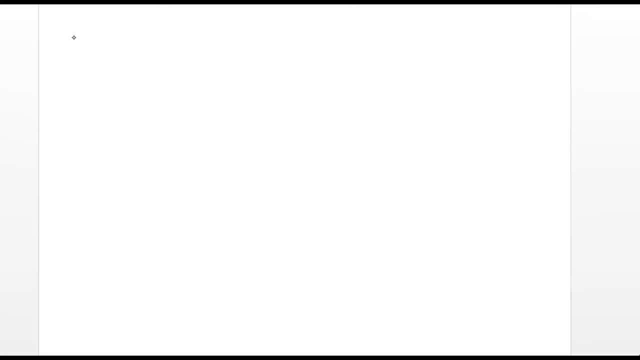 second for seepage velocity. so first we have to find out the dry density. so dry density equal to mass by volume. so that is mass of specimen divided by area into length, that is volume. so mass is a 495, that's a given areas, 50, that's also. 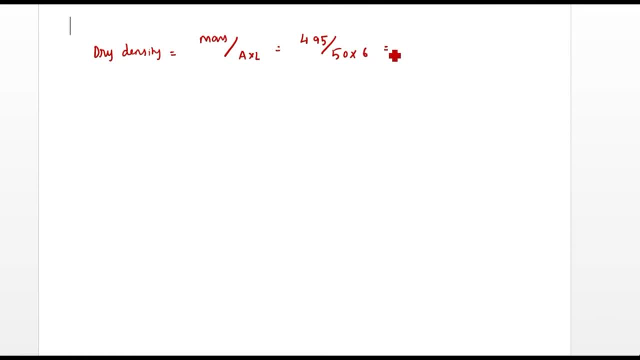 given into length of sample 6 is given. so from that we we can find out: zero point sorry. one point six, five gram per centimeter cube. okay, so now gamma D, equal to Rho D, into nine point eight one. so now Rho D is equal to one point. 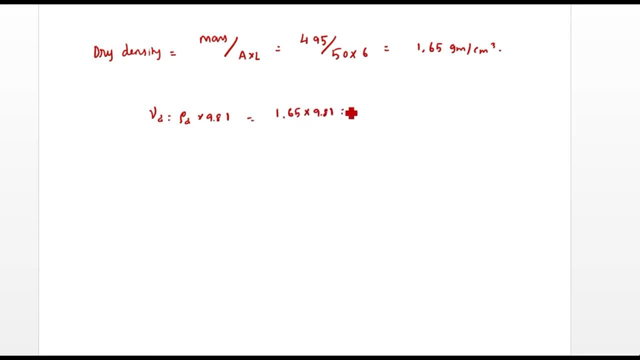 six five into nine point eight one. so we got the value of sixteen point one, eight six five. so now the settling velocity V s equal to V divided by n. okay, so now we have to find out the n value. so n value we can find out from gamma D. so gamma D. 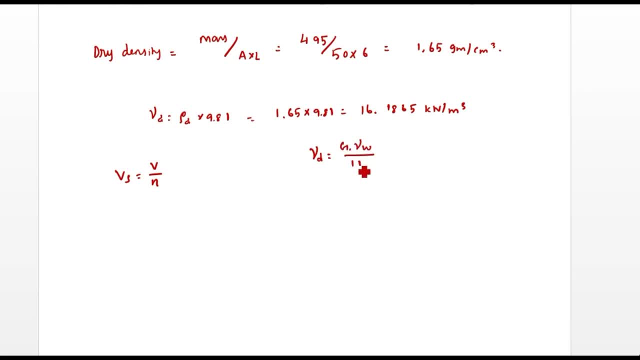 equal to G into gamma W divided by 1 plus e, N, which the value, the n, is equal to 0.05 N. so we can substitute all the values so gamma 2015.186 place equal to so G values. two point six muita gamma D is nine. 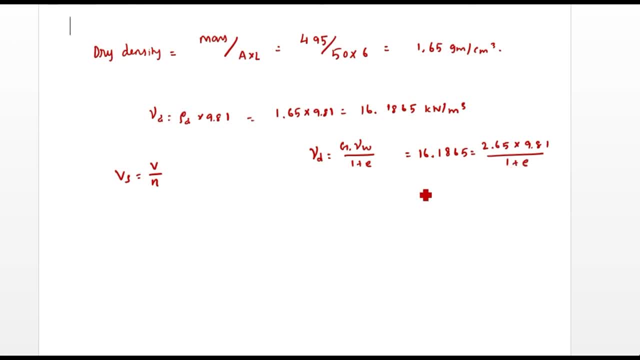 point eight, one divided by 1 plus e. so our only unowness he. so from that we can find out that e is equal to 0.60 six. okay, so now we you have to find out the n value. so from the e, so n value n. 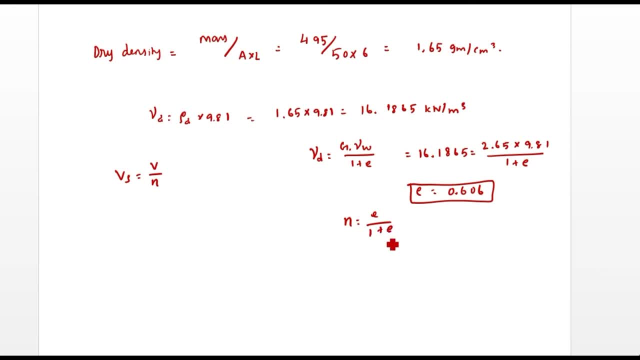 So N equal to E divided by 1 plus E. So this is a formula we know. So E equal to 0.606 divided by 1 plus 0.606, that is 1.606.. From that we got the value of 0.3773, that is 37.73 percentage. that is the N value. 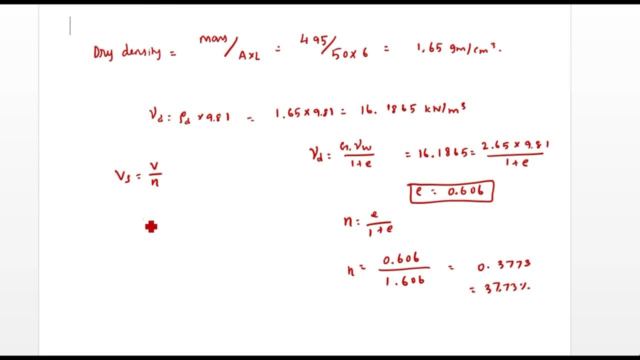 Okay, So now we can substitute all the values over here. So V is equal to 0.015. that is a given- Sorry, that is a that we find out- And N value is 0.3773.. So from that we got the value of 0.03975 centimeter per second. 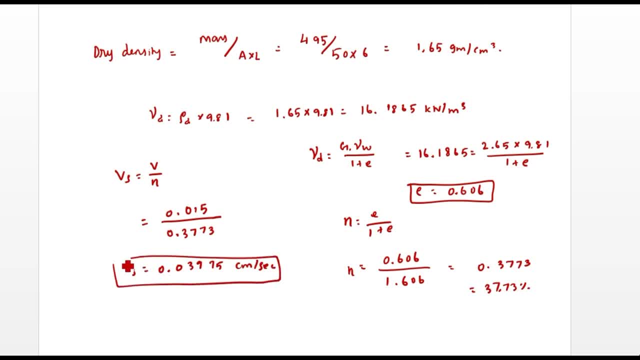 Okay, So this is the settling velocity. Sorry, this is the seepage velocity. So this is the method we can solve the problem. Again, we will see in next video. Thank you.